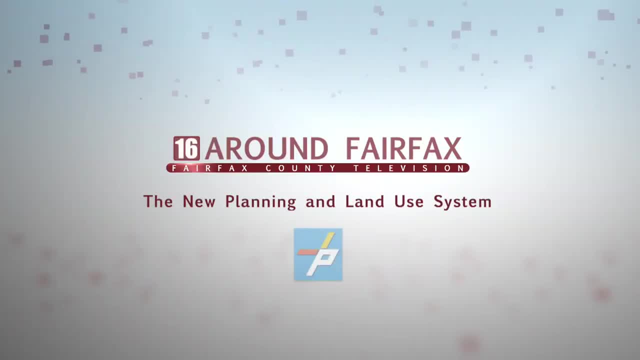 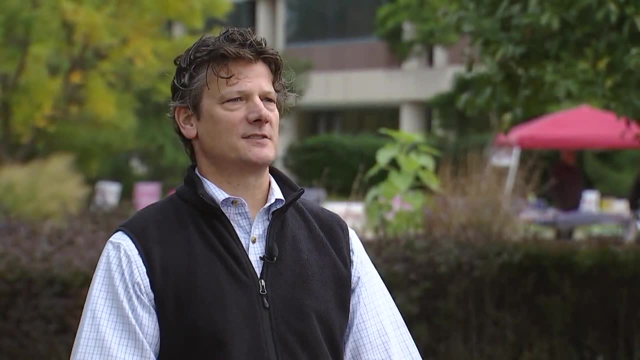 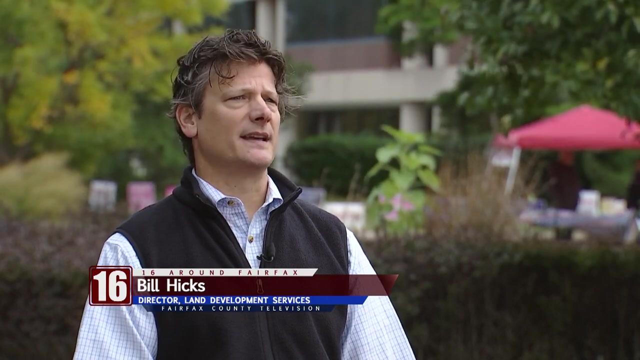 Plus is our new permitting and land use system. It'll be the single place for customers to come and apply for their permits, whether it's a building permit, a zoning permit, a land disturbance application, or even to file a complaint about a code violation. So Plus, 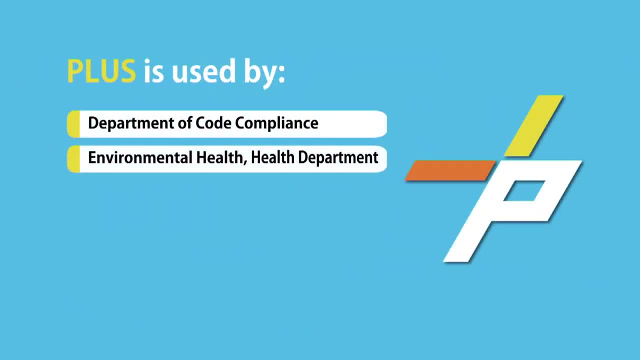 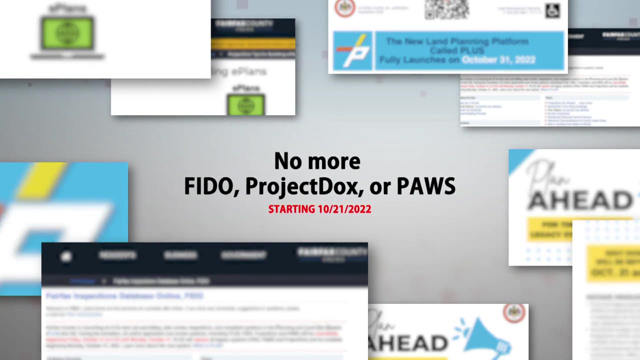 will be used by the Department of Code, Compliance, Environmental Health and the Department of Health, Planning and Development, the Office of the Fire Marshal and Land Development Services. The county is updating the system because currently we're using a variety of disparate systems that are fairly old, some as many as 20 or 25 years old. So we're moving to. 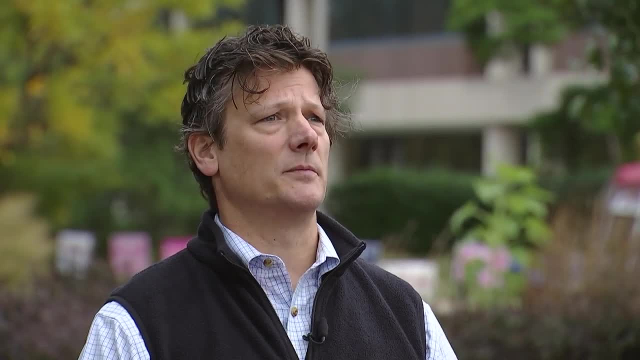 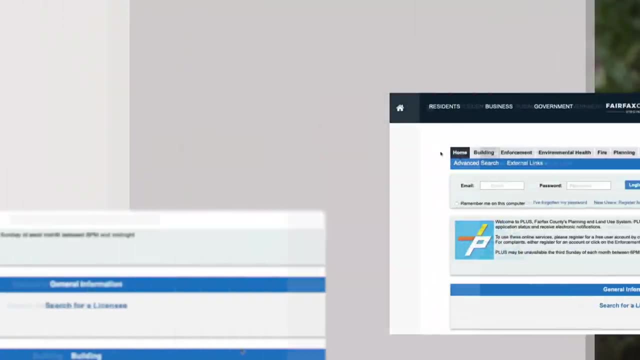 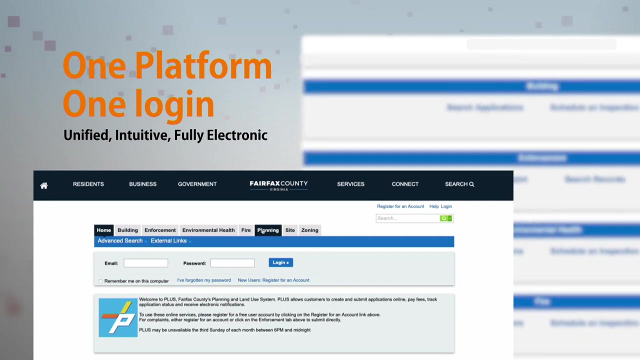 a place where these are new and modern technologies that will help our customers. It will allow for a single access, a single login for our customers and very unified and intuitive method to apply for these permits. And, frankly, moving to modern technology, allows us to be fully electronic, Electronic. 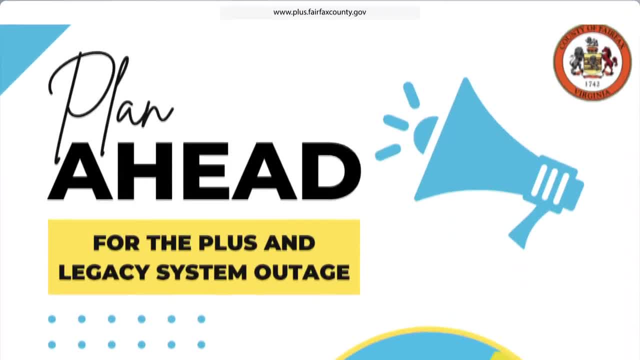 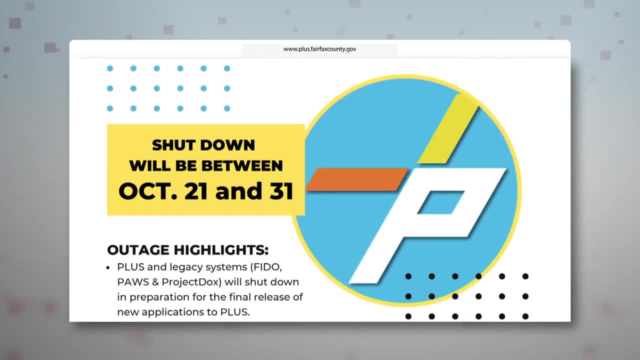 plan submittal, electronic permit application and electronic permit processing. This is going to happen on October 21st. We're bringing our old legacy systems down and installing the new system. then The new system will launch on Monday morning, October 31st, If you are. 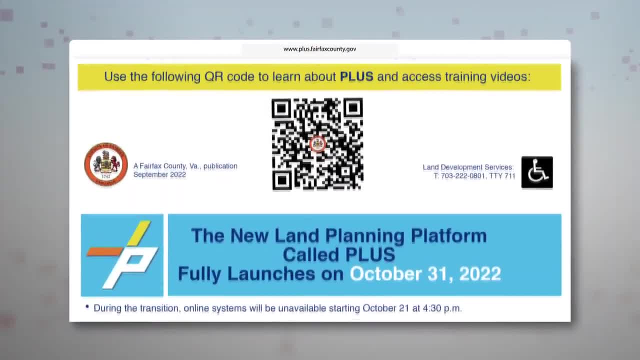 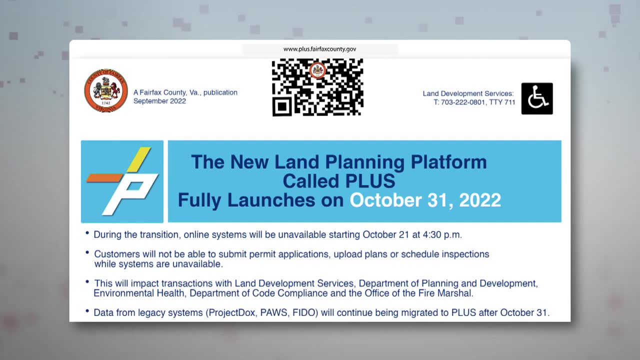 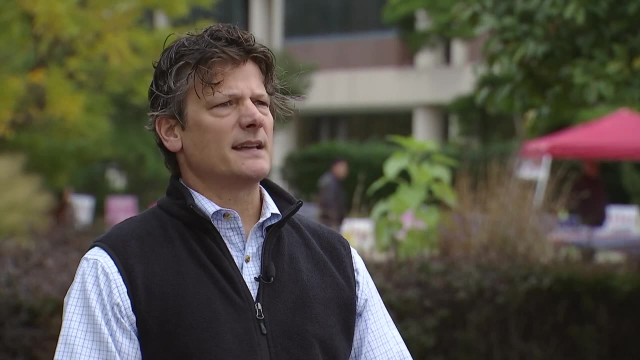 applying for a permit, you should plan to apply early. If you cannot get it done prior to the 21st, I recommend that you hold off until after the 31st and the new system is up and running. So if you submit right at October 21st, we will still have to migrate your data. It might. 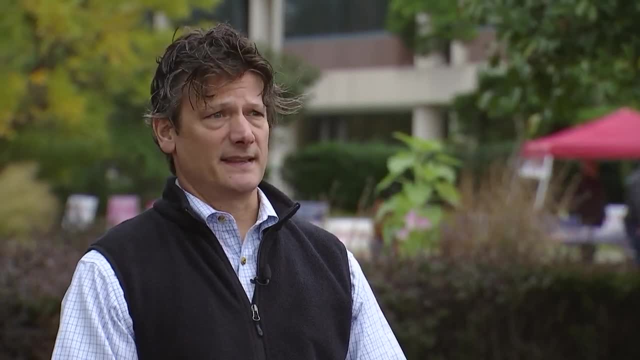 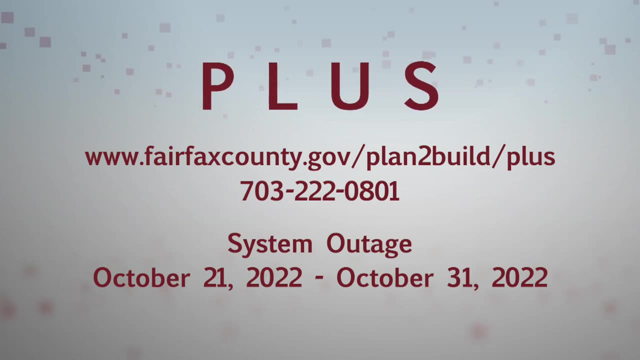 take a few more days, but our team is ready and able to serve to get that data moved over as quickly as possible. For more information, you should come to our website. We've got directions to our YouTube channel. We've got webinars. We're ready to help you at any point. 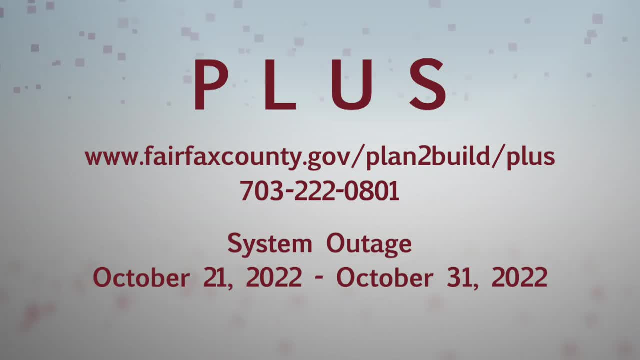 Our number is 703-222-0801.. For more information, visit wwwfemagov.